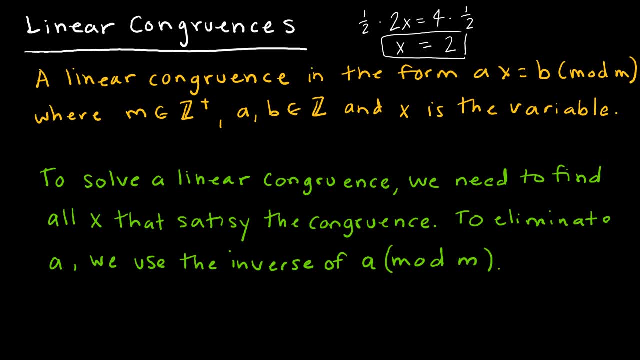 would be two and I would have just one solution, because it's a linear equation. Now we're dealing with a linear congruence: ax equals b mod m And essentially what we're saying is we have to find the inverse of a and we're going to find the inverse of b mod m. So we're going to find the 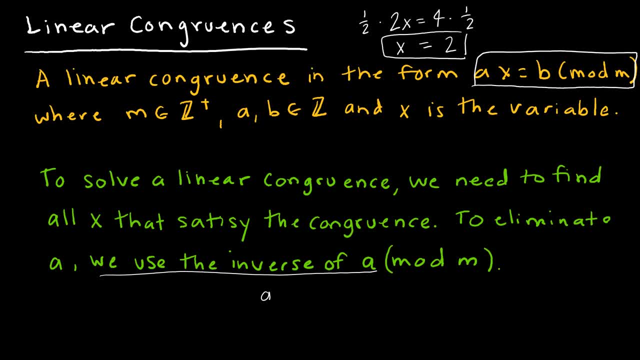 inverse of a and we're going to find the inverse of a and we're going to find the inverse of a- a, so that if I take a inverse which we're going to denote with a line over it, times a- x equals a, inverse times b mod m, then on the left side I'm just going to be left with. 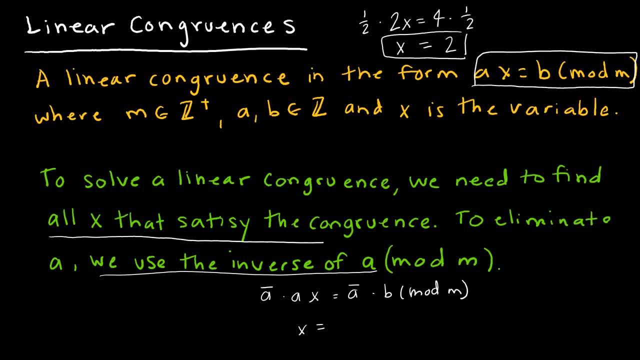 x equals, and that's what I'm doing- is trying to find all of the x's that satisfy the congruence. So I'm solving for x On the right side. I'm going to have some value, mod m Now keep in mind. 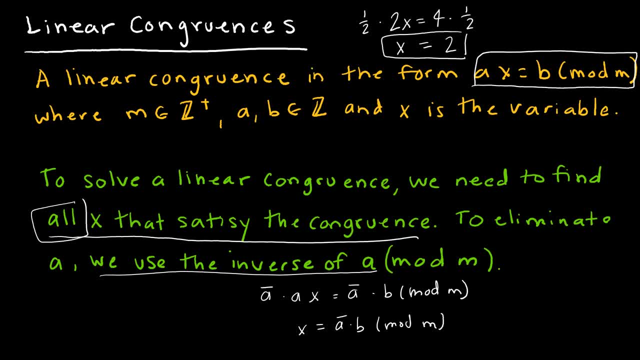 we said we need to find all of the x's. so we know with modular arithmetic that any value that has the same remainder is going to be the same equivalent value, mod m. So that's what we're doing, is finding a value, mod m, and then we're going to continue to find more values based on. 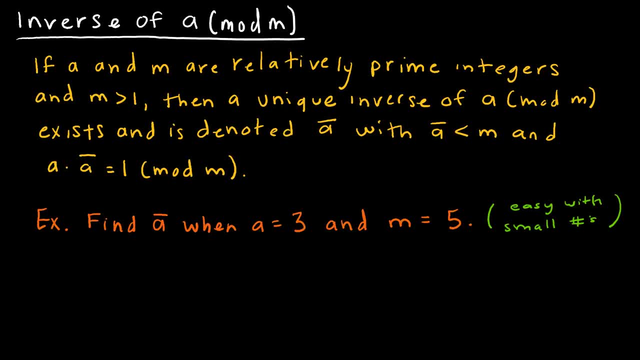 that original value. We're going to start by first learning how to find the inverse, which can be complicated. So I'm going to show you a very easy example and then a more complicated example, and then we're going to talk about how to use the inverse to solve the linear congruence. So this is just 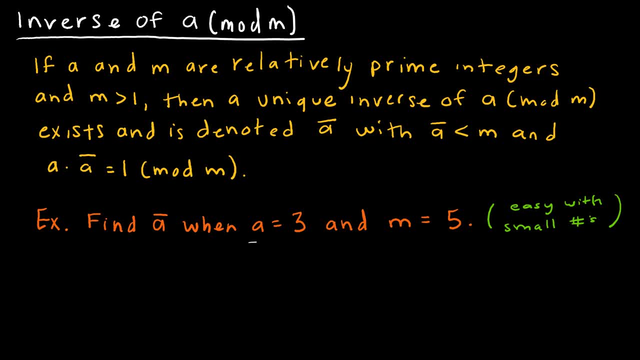 finding the inverse. So we're saying: if a and m, a and m are relatively prime, and you'll recall that means they don't have any factors in common, and m is greater than one, so the mod of m is greater than one. and so if a and m are relatively prime, and you'll recall that- 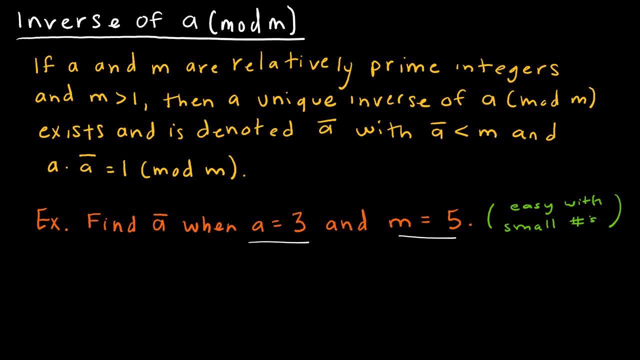 that we are in, the modulo that we are in, is greater than 1, that a unique inverse of a mod m exists and is denoted with the a bar, where obviously a bar is less than m and obviously the most important part, which we've just talked about, is a times a inverse is 1 mod m, which is 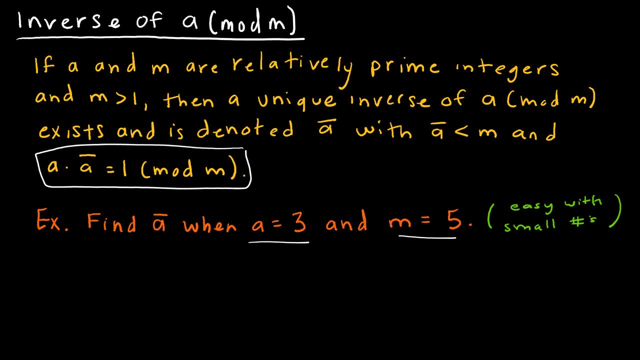 why we want to find it. So. when we're dealing with small numbers like this, essentially what I can do is I can say 3 times some number. 3 being a is equal to my mod times some number plus 1.. Now why did I choose 1? Because I want the solution to be 1, which means I want the remainder. 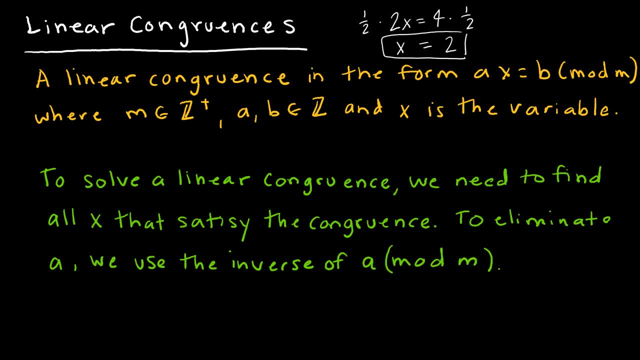 be 2, and I would have just one solution, because it's a linear equation. Now we're dealing with linear congruence: ax equals b mod m And essentially what we're saying is we have to find the inverse of a, so that if I take a inverse which we're going to denote with a line over it, 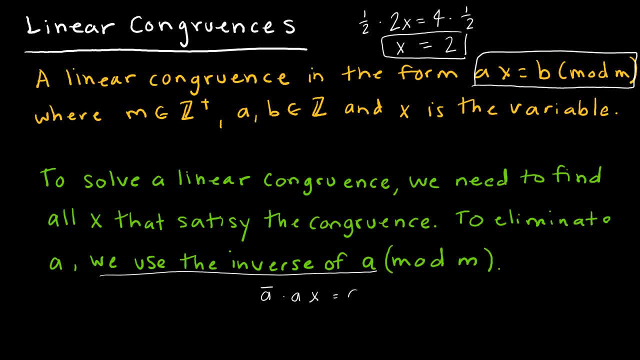 times a, x equals a. inverse times b mod m. then on the left side, I'm just going to be left with x equals, and that's what I'm doing- is trying to find all of the x's that satisfy the congruence. 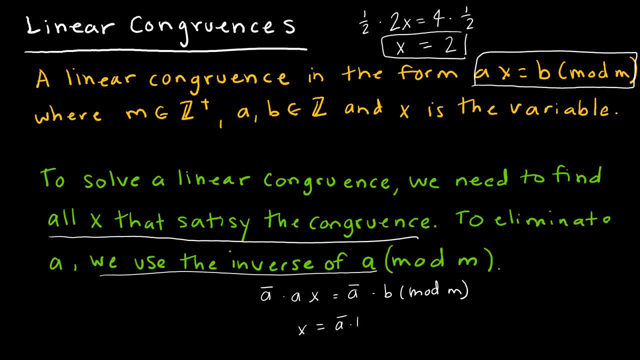 So I'm solving for x On the right side I'm going to have some value mod m. Now keep in mind we said we need to find all of the x's, so we know with modular arithmetic that any value that has the same remainder is going to be the same equivalent value mod m. So that's what we're. 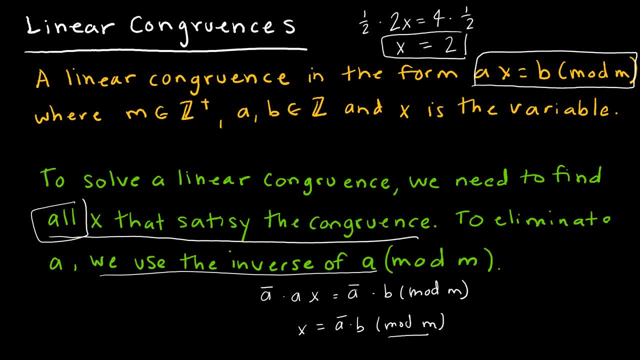 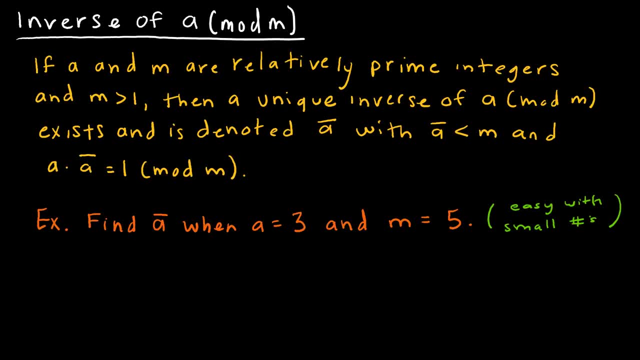 doing is finding a value- mod m- and then we're going to continue to find more values based on that original value. We're going to start by first learning how to find the inverse, which can be complicated. So I'm going to show you a very easy example and then a more complicated example, and then we're 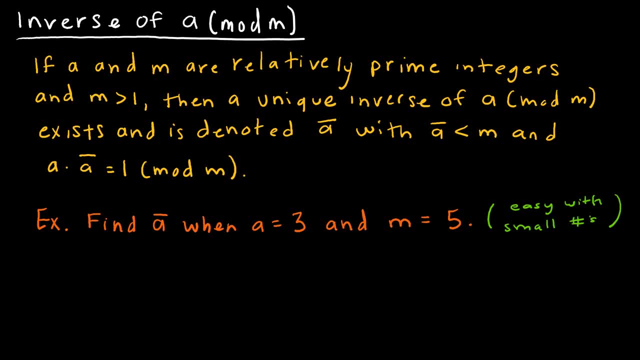 going to talk about how to use the inverse to solve the linear congruence. So this is just finding the inverse. So we're saying, if a and m, a and m are relatively prime, and you'll recall that means they don't have any factors in common and m is greater than 1, so the mod of b 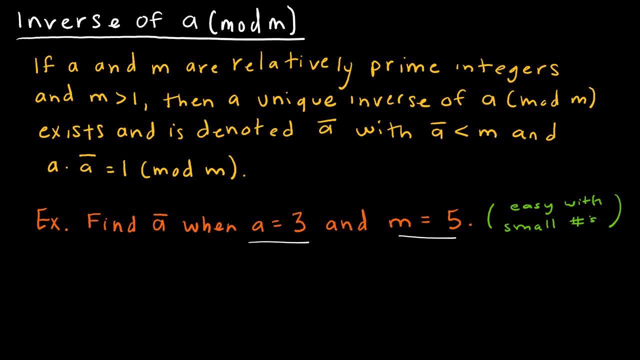 that we are in, the modulo that we are in, is greater than 1, that a unique inverse of a mod m exists and is denoted with the a bar, where obviously a bar is less than m and obviously the most important part, which we've just talked about, is a times a inverse is 1 mod m, which is 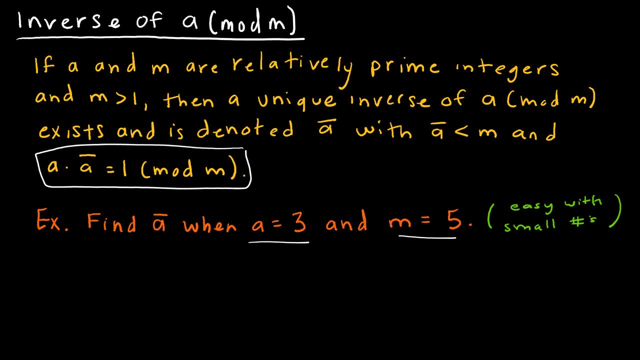 why we want to find it. So. when we're dealing with small numbers like this, essentially what I can do is I can say 3 times some number. 3 being a is equal to my mod times some number plus 1.. Now why did I choose 1? Because I want the solution to be 1, which means I want the remainder. 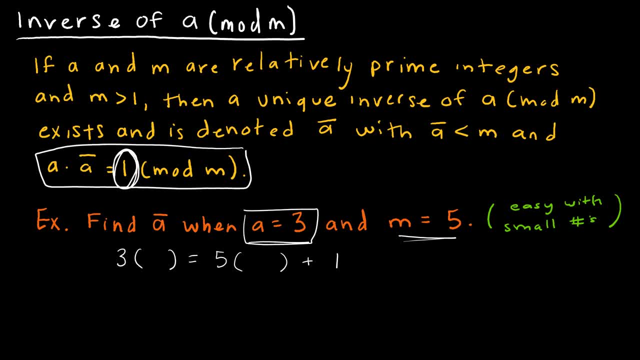 in mod m to be 1.. So if I take 5 times something and we're in mod 5, then 5 times m is equal to mod m. So if I take 5 times something and we're in mod 5,. 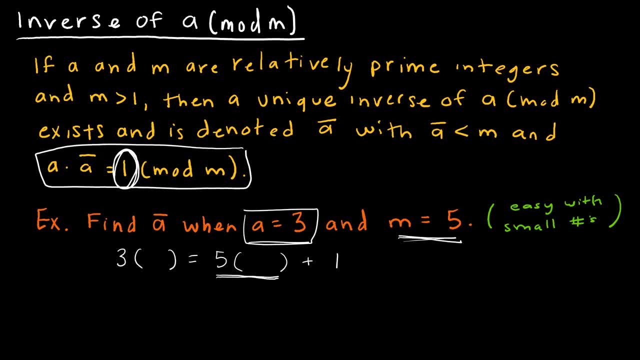 then 5 times m is equal to mod m. So if I take 5 times something and we're in mod 5,, 5 times something plus 1 would obviously be congruent to 1 mod 5.. Again, because 5 times something, this would be 0 mod 5, plus 1 would make it 1 mod 5,. 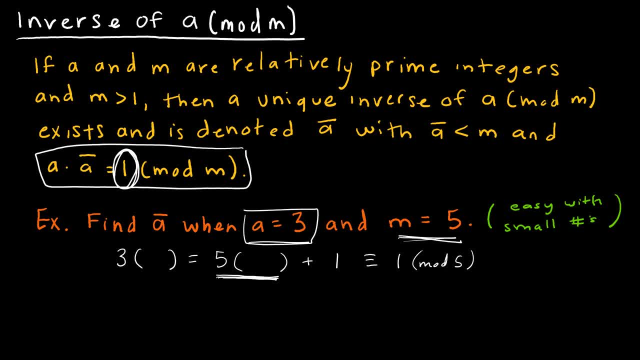 because that's the remainder. So I'm just going to do some plugging in and just seeing what I can come up with. So let's start with 1, 5 times 1.. 5 times 1 is 5, plus 1 is 6, and can I find? 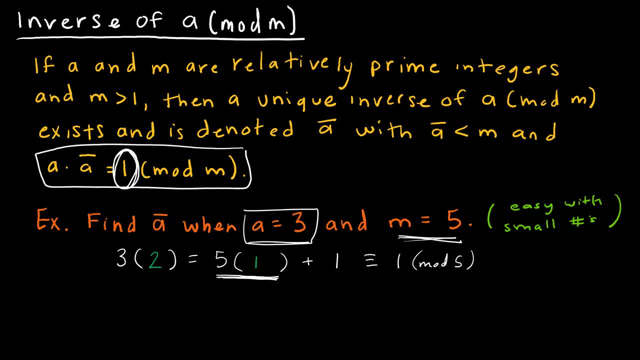 an integer value here that equals 6?? Yes, I can. So in fact I have just found the inverse is 2.. So you might be thinking: well, that was way too easy, So think about if I tried this again. 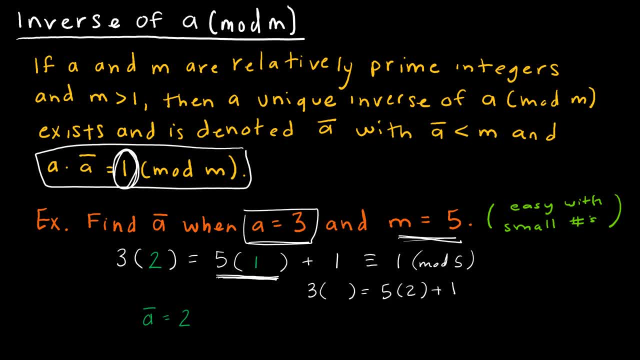 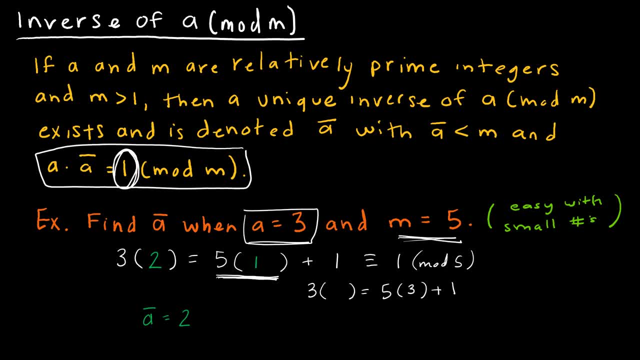 15 plus 1 is 16.. Again, I can't find an integer value for using 3. And I could try it again for 4.. 5 times 4 is 20.. 20 plus 1 is 21.. And I could find 1 for 4, which is 7.. But what I'm looking for 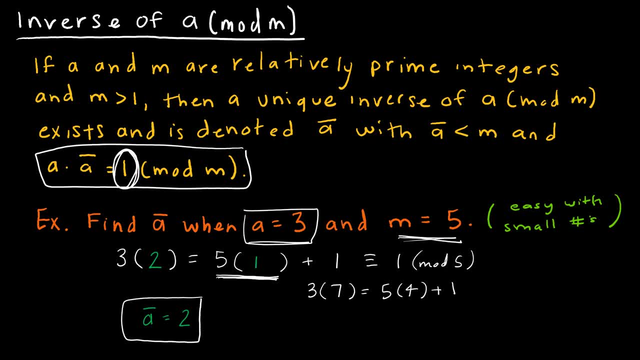 is that A inverse to be obviously the smallest value? So, because I'm in mod 5, 7 is going to work, And then if I add another 5 to that, 12 is going to work. So I'm going to add another 5 to. 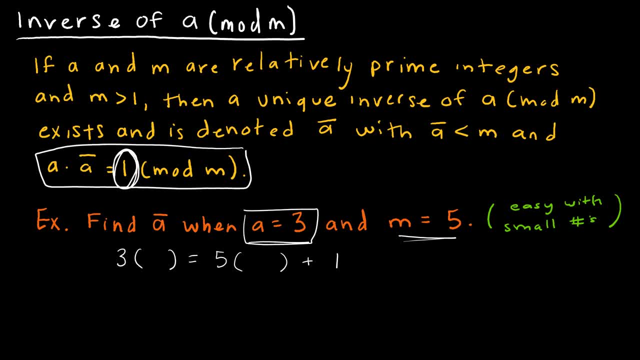 in mod m to be 1.. So if I take 5 times something and we're in mod 5, then 5 times m is equal to mod m. So if I take 5 times something and we're in mod 5,. 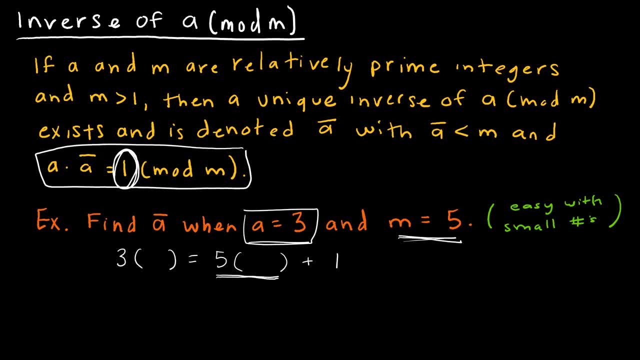 then 5 times m is equal to mod m. So if I take 5 times something and we're in mod 5,, 5 times something plus 1 would obviously be congruent to 1 mod 5.. Again, because 5 times something, this would be 0 mod 5, plus 1 would make it 1 mod 5,. 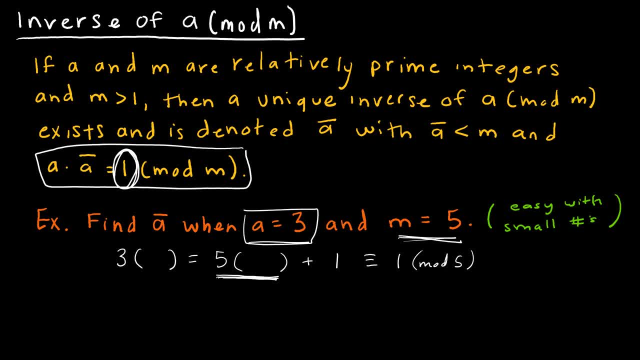 because that's the remainder. So I'm just going to do some plugging in and just seeing what I can come up with. So let's start with 1, 5 times 1.. 5 times 1 is 5, plus 1 is 6, and can I find? 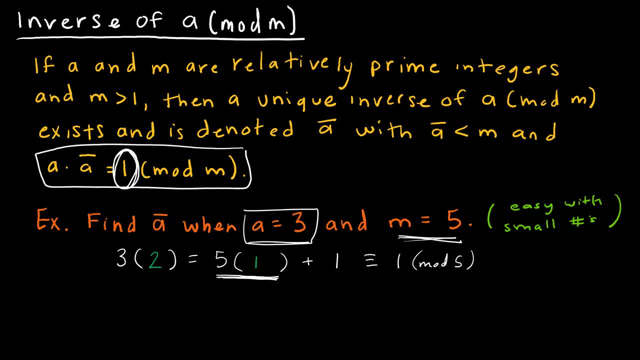 an integer value here that equals 6?? Yes, I can. So in fact I have just found the inverse is 2.. So you might be thinking: well, that was way too easy, So think about if I tried this again. 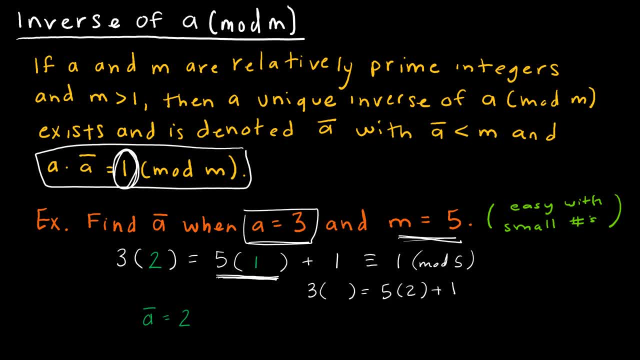 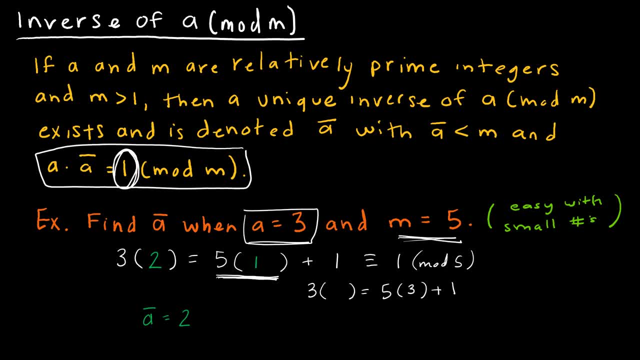 15 plus 1 is 16.. Again, I can't find an integer value for using 3. And I could try it again for 4.. 5 times 4 is 20.. 20 plus 1 is 21.. And I could find 1 for 4, which is 7.. But what I'm looking for 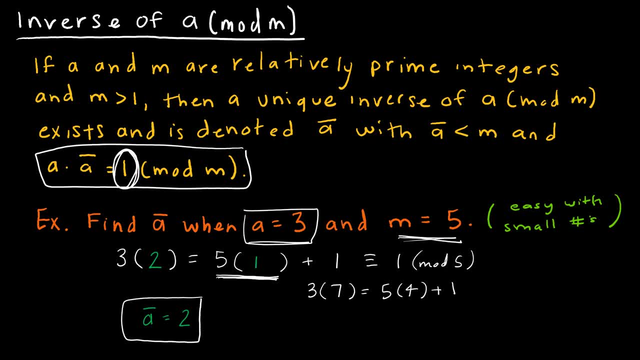 is that a inverse to be obviously the smallest value? So, because I'm in mod 5, 7 is going to work, And then if I add another 5 to that, 12 is going to work. So I'm going to add another 5 to. 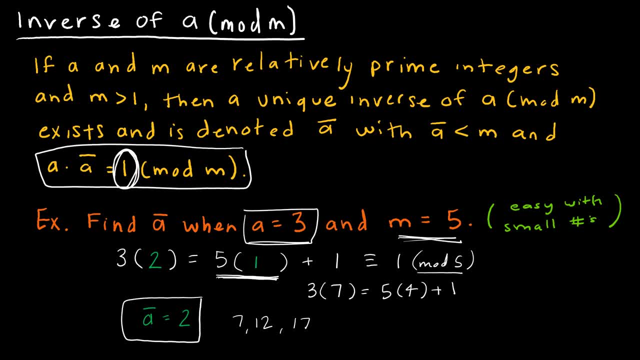 that 17 is going to work, And if I subtracted 5 to get 2 minus 5 is negative 3 and negative 8, all of those are going to work. But what I'm looking for is just that first value. But 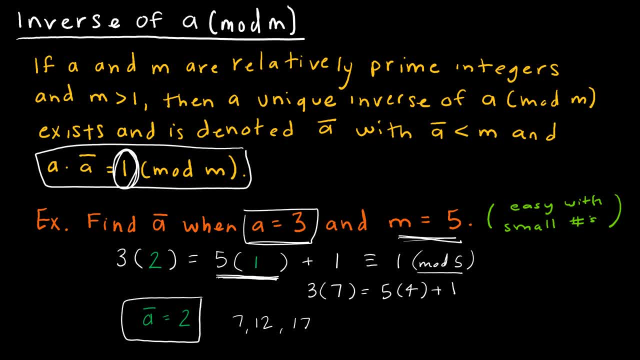 that 17 is going to work. And if I subtracted, you know, 5 to get 2 minus 5 is negative 3 and negative 8.. All of those are going to work, But what I'm looking for is just that first value. 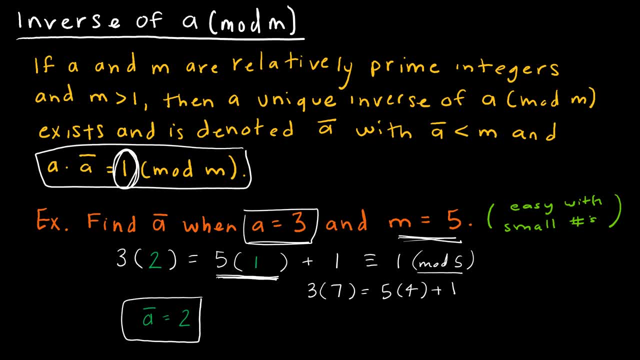 But obviously this only works for small numbers And it seems a little silly because it's just sort of a guess and check method. So now let's look at how we actually will solve to find the inverse. In this example, we are going to find the inverse of 2.. So we're going to find the inverse of 2.. 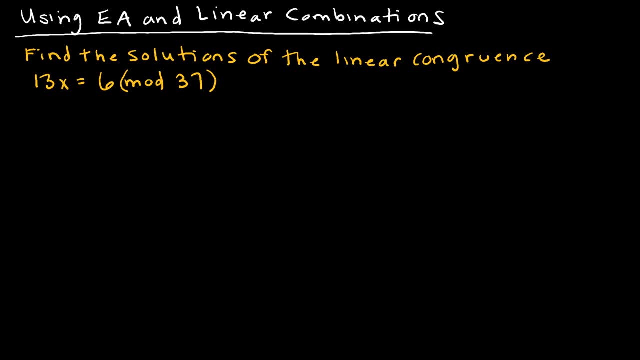 And then we're going to go through a full example. So not only are we going to find the inverse, which is going to be far more complicated on this example, because we can't just guess and check- We're going to use the Euclidean algorithm and linear accommodations, Then we're going to 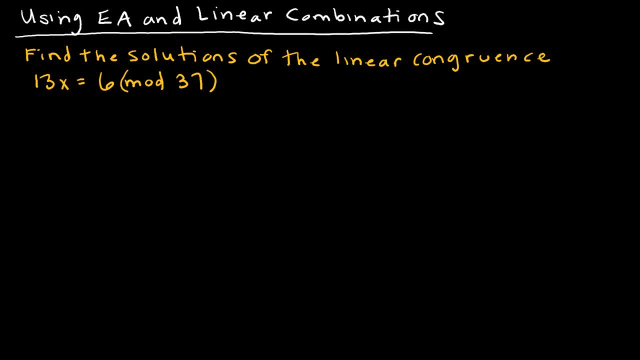 use that to actually find the solutions, which we did not do in the last example. All we did was find the inverse. So there's going to be a lot going on here, So try to keep yourself as organized as possible. The first step is that we have to organize the solutions. So we're going to 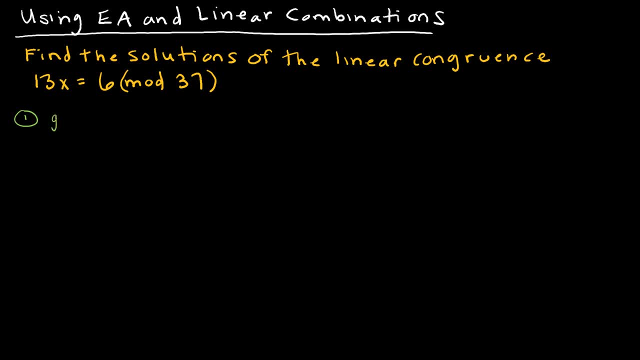 of course, find the inverse, But in order to do that, I have to first show that the GCD of 37,, which is my mod, and 13,, which is my A value- remember AX- equals. I need to show that that is equal to 1.. The reason I 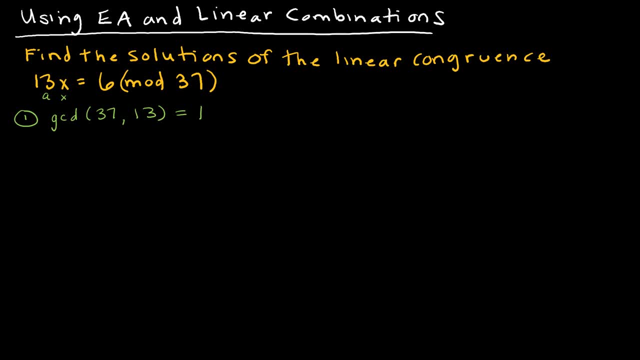 have to do that is because we have to show that these are relatively prime. So let's start using the Euclidean algorithm. So hopefully you've already watched that video and know how this works. Otherwise this might be super confusing for you. I'm going to write 37 as a product of 13 and some number- in this case 2, with some. 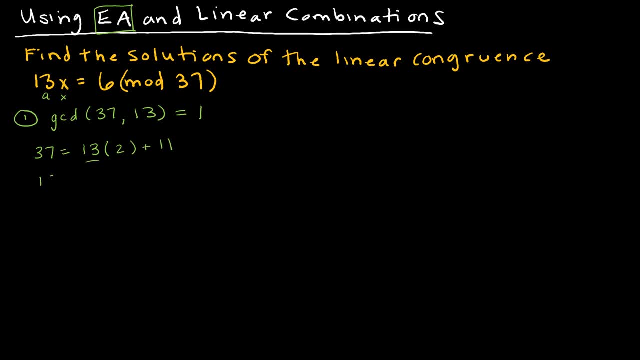 remainder. Then I'm going to take the quotient of 13 and the remainder of 11 and repeat the process, And then the quotient of 11 and the remainder of 2 and repeat the process, And the quotient of 2 and the remainder of 1 and repeat the process, And I keep going until I no longer. 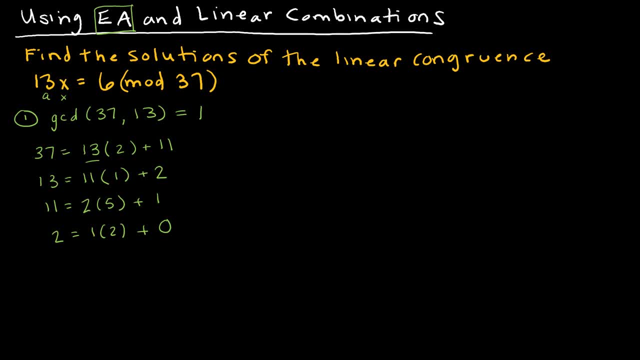 have a remainder, and whatever the remainder was before, 0 is my GCD. So I have in fact verified that the GCD is 1.. Step two is that I have to write the value as a linear combination, And, again, we've already learned how to do. 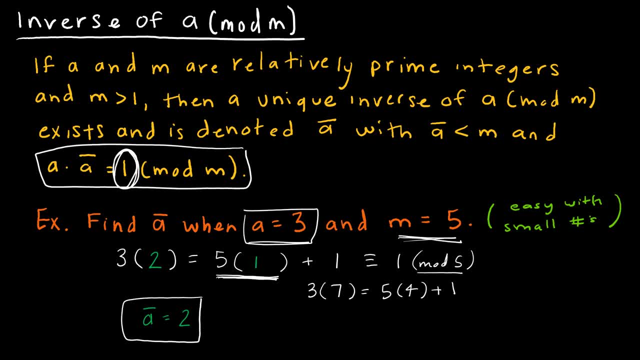 obviously this only works for small numbers And it seems a little silly because it's just sort of a guess and check method. So now let's look at how we actually will solve to find the inverse In this example. we are going to solve for the inverse, So we're going to find the 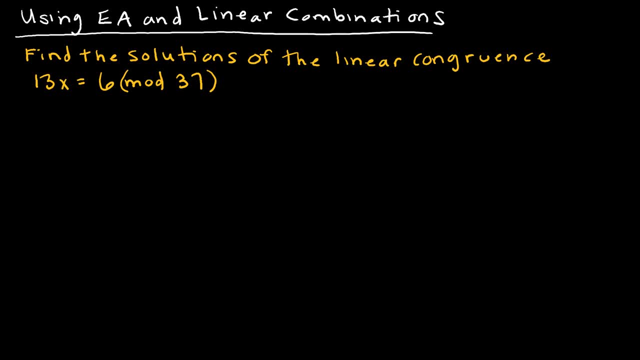 inverse, And then we're going to go through a full example. So not only are we going to find the inverse, which is going to be far more complicated on this example, because we can't just guess and check- We're going to use the Euclidean algorithm and linear accommodations. 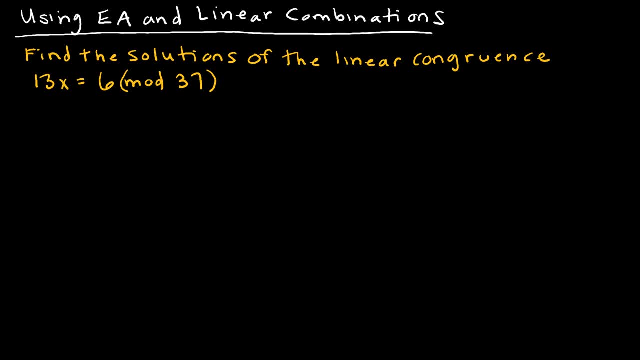 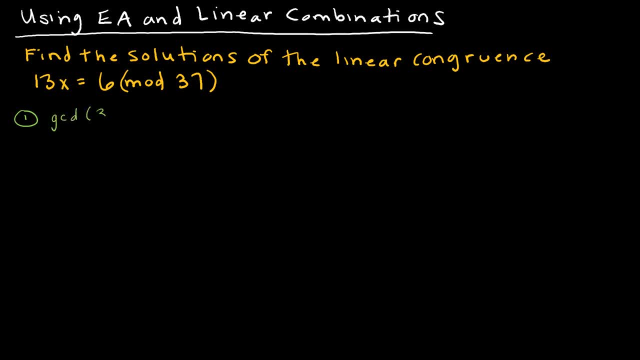 I have to first show that the GCD of 37,, which is my mod, and 13,, which is my A value- remember AX- equals. I need to show that that is equal to 1.. The reason I have to do that is because we have 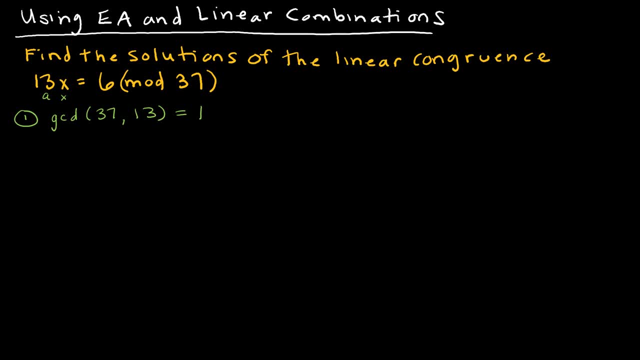 to show that these are relatively prime. So let's start using the Euclidean algorithm. So hopefully you've already watched that video and know how this works. Otherwise this might be super confusing for you. I'm going to write 37 as a product of 13 and some number, in this case 2,. 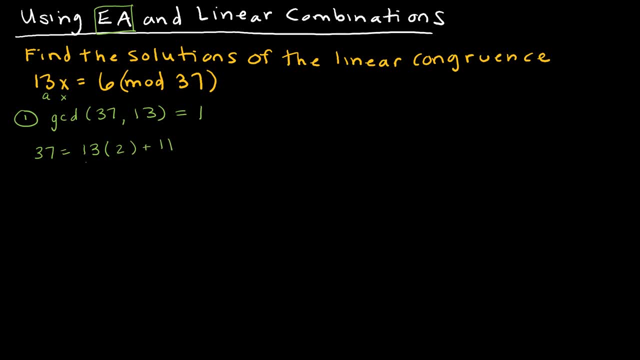 with some remainder. Then I'm going to take the quotient of 13 and the remainder of 11 and repeat the process, And then the quotient of 11 and the remainder of 2 and repeat the process, And the quotient of 2 and the remainder of 1 and repeat the process, And I keep going until I no longer. 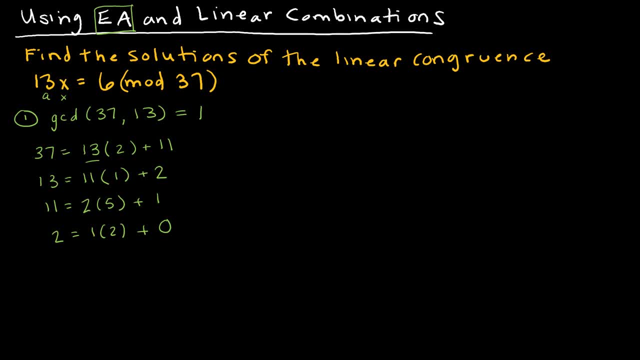 have a remainder, And whatever the remainder was before, 0 is my GCD. So I have in fact verified that the GCD is 1.. Step 2 is that I have to write the value as a linear combination And again, we've already learned how to do this, but it's kind of a lot of work. So we started by saying: 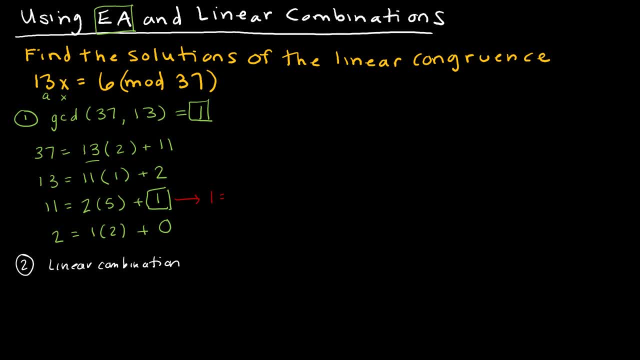 so when I write my three basic equations, I'm going to first change what Iщ will be written as your GCD. I'm going to have two of those as my GCD and one the��� piece plus theìs piece- And then give it a slight change of magnitude to Euclidean and write this out and rewrite it. 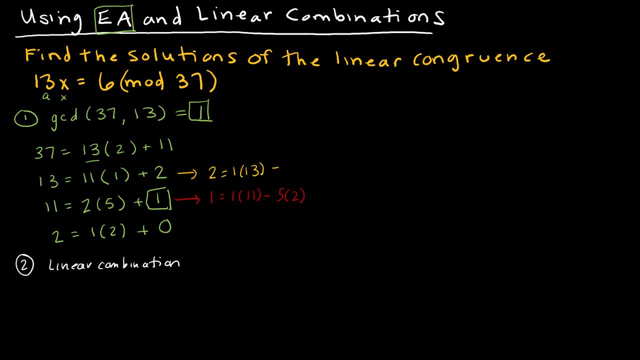 as one equals, and then one times eleven minus two times five, or I'm going to write five times two, And then this guy is going to be rewritten as 2 equals one times thirteen minus one times eleven, And then this guy is going to be rewritten as four times. Now, if you look here from the R prayer: 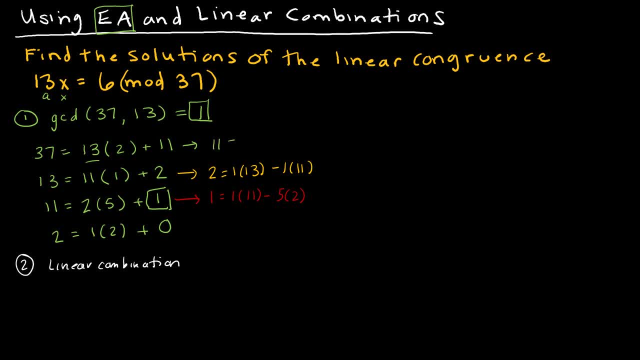 you'll have the most waist-to-ta chopping be seen. And then what we've learned in the contract is that the position G takes one from. x equals future term and frequently the favourites work, So as 11 equals 1 times 37 minus 2 times 13.. 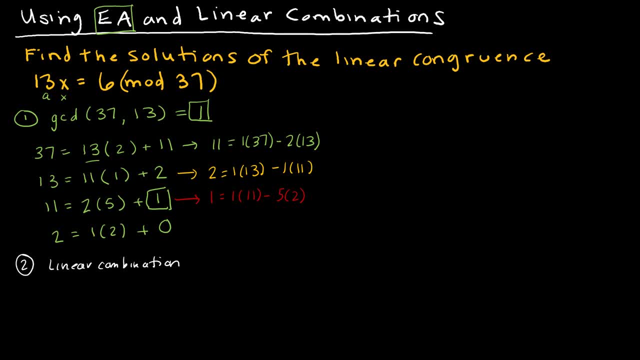 And then I'm going to take my first one: 1 equals, because that's what I want- is 1 equals, and I'm going to rewrite it and instead of 2, I'm writing the expression that is equal to 2.. 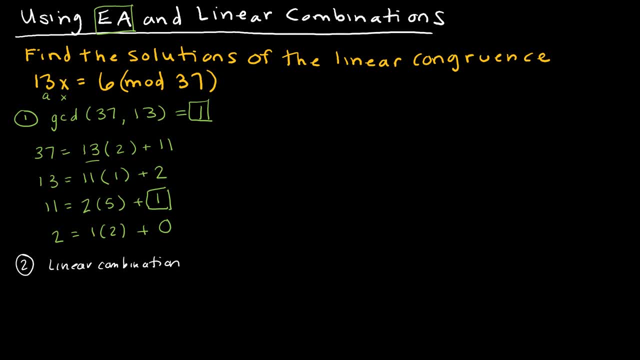 this, but it's kind of a lot of work. So we started by saying: let's take this guy And rewrite it as 1 equals, and then 1 times 11 minus 2 times 5.. Or I'm going to write 5 times 2.. 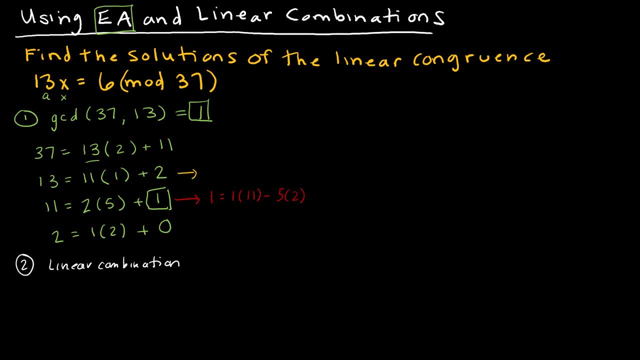 And then this guy is going to be rewritten as 2 equals 1 times 13 minus 1 times 11.. And then this guy is going to be rewritten as 11 equals 1 times 37 minus 2 times 13.. And then I'm going to take my first one: 1 equals, because that's what I want, is 1 equals. 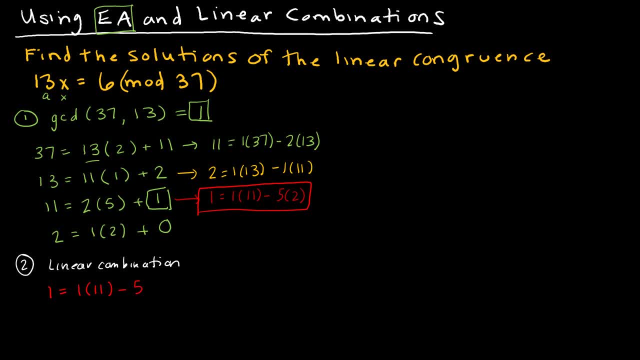 And I'm going to rewrite it, And instead of 2, I'm writing the expression that is equal to 2.. So 5 times 1 times 13, minus 1 times 11.. And then recall- I'm looking just for how many groups of each- 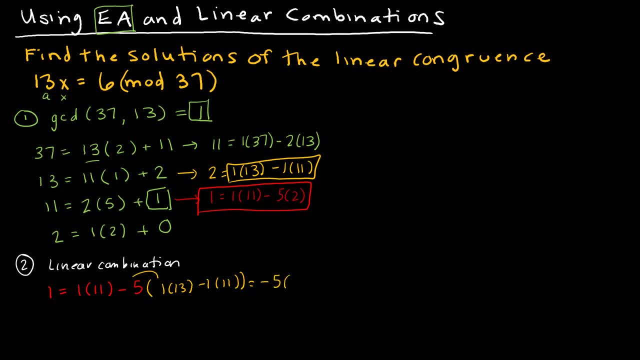 So I have negative 5 times 1,, so I have negative 5 groups of 13.. And then negative 5 times negative. 1 is positive 5 plus 1, which is 6 groups of 11.. And now I'm going to replace 11 with all of the things that 11 is equal to. 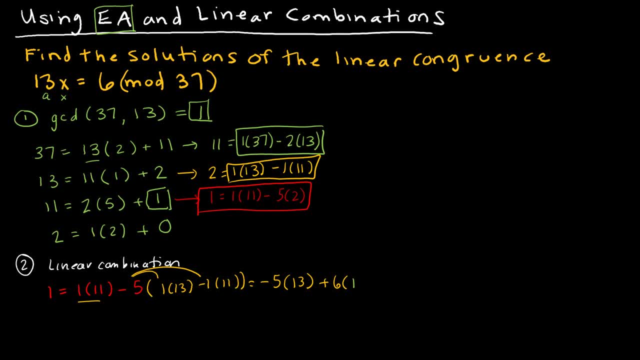 So I'm just going to cheat and write: 1 times 37 minus 2 times 13. And that gives me 6 times 1, or 6 groups of 37. And then 6 times negative- 2 is negative- 12 groups of 13,. 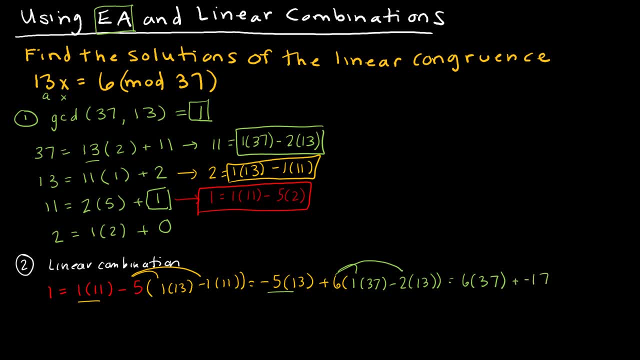 plus another negative 2. 5, so that's negative 17 groups of 13.. So that is my linear combination. So what am I going to do with that? Well, step 3 says: once you have your linear combination which, as we recall, is 1, equals. 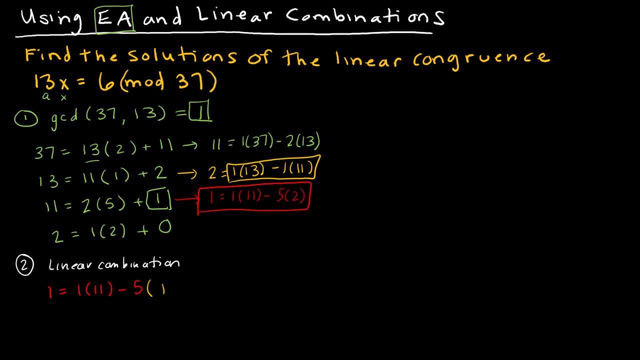 So 5 times 1 times 13, minus 1 times 11.. And then recall- I'm looking just for how many groups of each. So I have negative 5 times 1, so I have negative 5 groups of 13.. 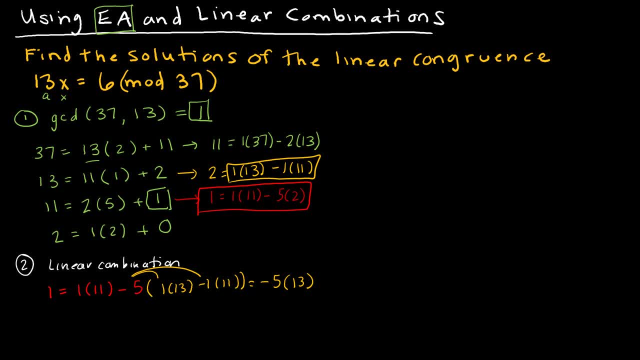 And then negative 5 times negative. 1 is positive, 5 plus 1, which is 6 groups of 11.. And then I'm going to take my first one, and now I'm going to replace 11 with all of the things that 11 is equal to. 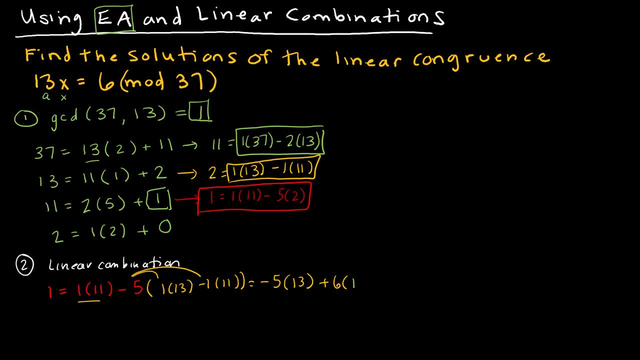 So I'm just going to cheat and write: 1 times 37 minus 2 times 13. And that gives me 6 times 1, or 6 groups of 37. And then 6 times negative- 2 is negative- 12 groups of 13. 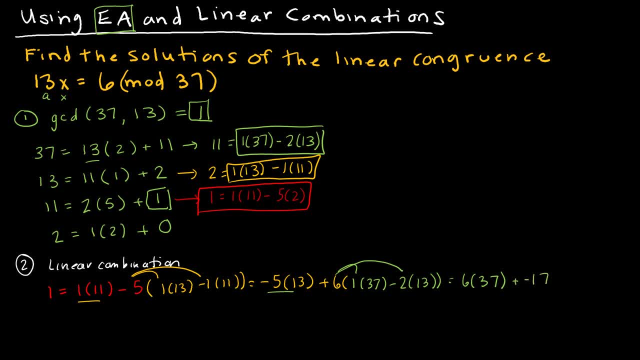 plus another negative 5.. So that's negative 17 groups of 13.. So that is my linear combination. So what am I going to do with that? Well, step 3 says: once you have your linear combination which, as we recall, is 1 equals 6 times 37.. 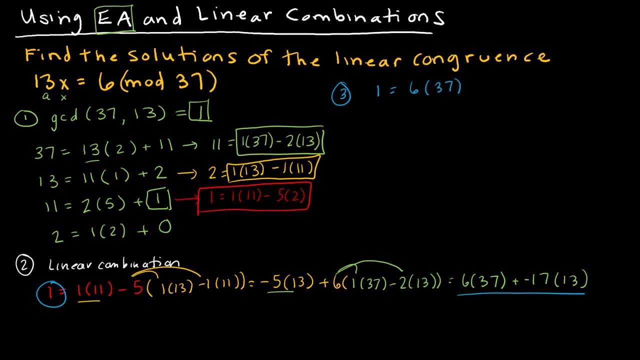 So 1 equals, and then all of this 6 times 37,, plus negative 17 times 13.. And keep in mind, all of this is in mod 37. So what I know about mod 37 is that 6 times 37,. 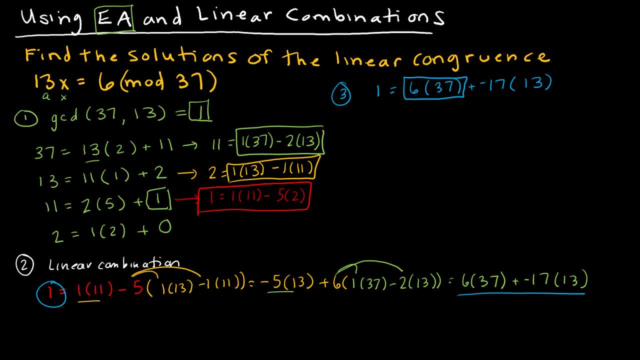 or any multiples of 37, essentially is going to be equivalent to 0 mod 37,, because they would have a remainder of 0. So what I'm looking for is that 1, is equivalent to negative 17 times 13 mod 37.. 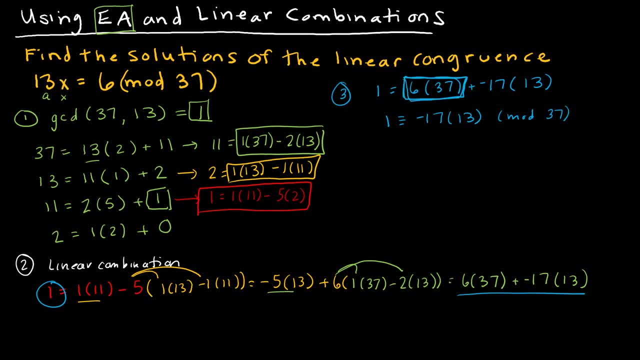 Because why did I just get rid of this? Because 6 times 37 is some value that is divisible evenly by 37. And so therefore, it is 0 mod 37. So I just got rid of it. So what did that do for me? 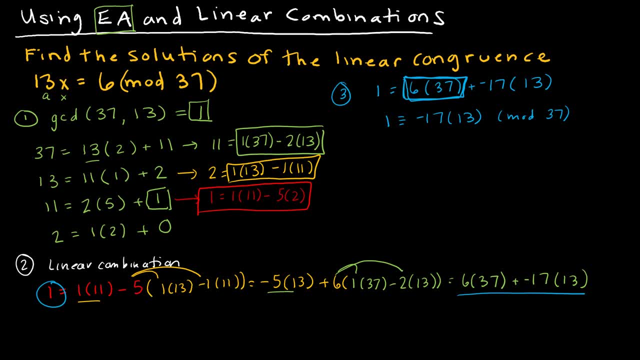 Well, that told me, which is the whole point- is that this guy is my inverse. So negative 17 is my inverse, because when I take it times 13,, I get 1.. So now, what am I going to do with that? 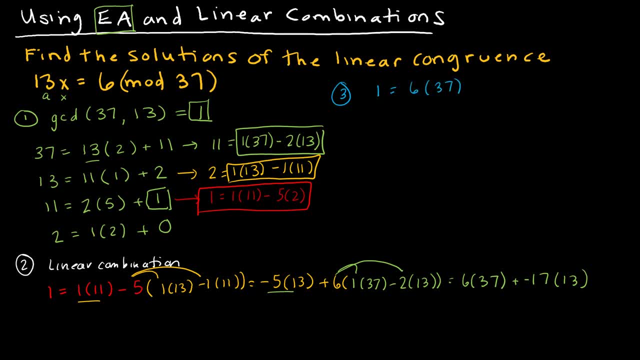 6 times 37. So 1 equals, and then all of this 6 times 37, plus negative 17 times 13.. And keep in mind, all of this is in mod 37. So what I know about mod 37 is that 6 times 37,. 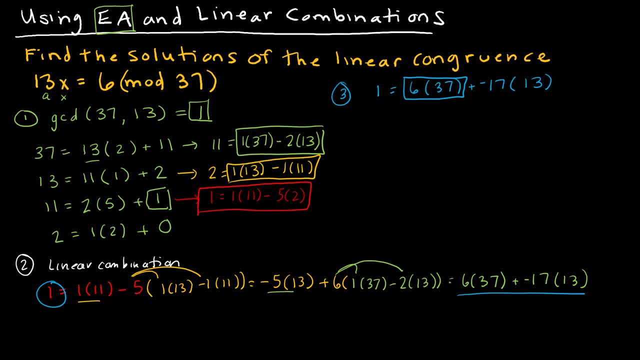 or any multiples of 37, essentially is going to be equivalent to 0 mod 37. Because they would have a remainder of 0. So what I'm looking for is that 1 is equivalent to negative 17 times 13 mod 37. Because why did I just get rid of this? Because 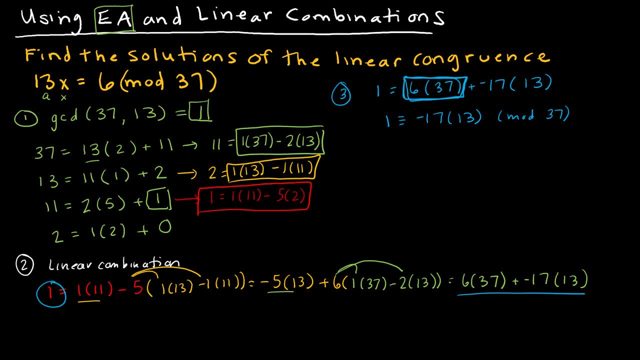 6 times 37 is some value that is divisible evenly by 37. And so, therefore, it is 0, mod 37. So I just got rid of it. So what did that do for me? Well, that told me, which is the whole point- is that this guy is my inverse. 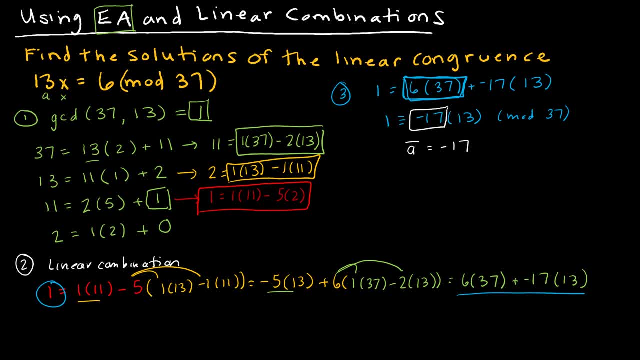 So negative 17 is my inverse, because when I take it times 13,, I get 1.. So now, what am I going to do with that? The most important step, and what we haven't done, is to find the solutions is I'm going to take. 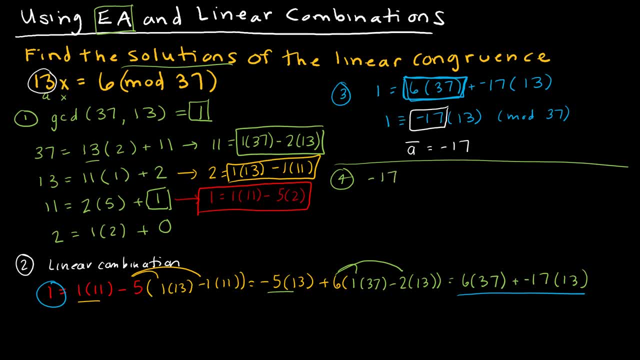 negative 17 times 13x. and then I'm going to take negative 17 times 6 mod 37. So what I know is that negative 17 times 13 is equal to 1, is congruent to 1 mod 37. So I've already shown it here, so I'm not going to show it again. I'm just going to say this side is x. Now the other side: if I take negative 17 times 13,, I get negative 102 mod 37. So now let's talk about the solutions. 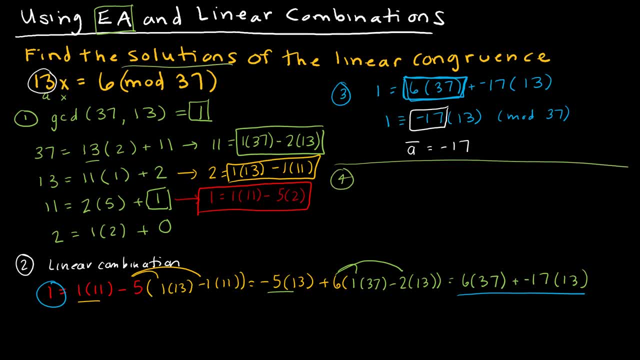 The most important step- and what we haven't done is to find the solutions- is: I'm going to take negative 17 times 13x and then I'm going to take negative 17 times 6 mod 37. So what I know is that negative 17 times 13 is equal to 1..